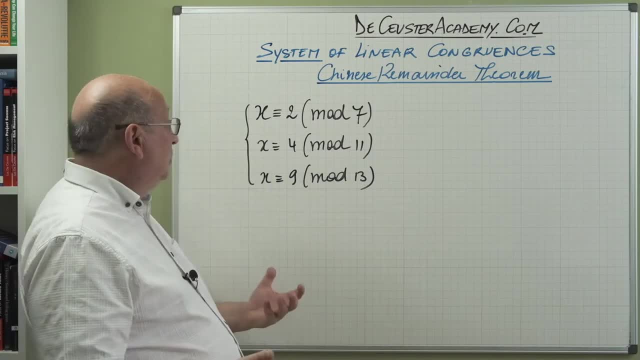 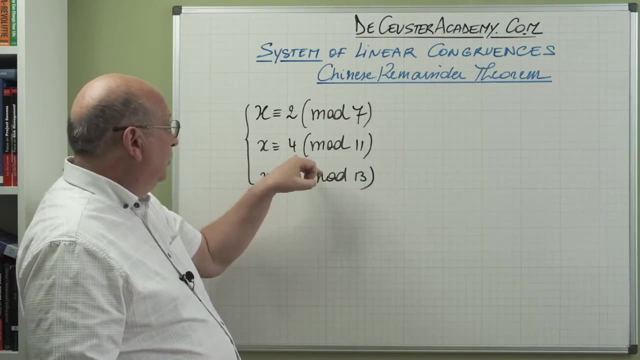 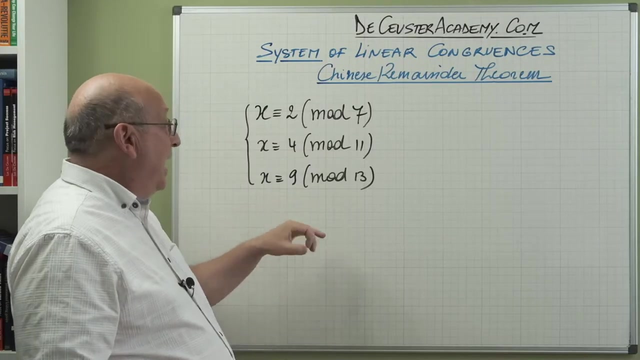 Basically, it means we're looking for a number X which, when we divide it by 7, the remainder is 2.. When we divide X by 11, we have a remainder of 4, and when we divide X by 13, the remainder is 9.. Let's now go through the different steps like we did before. First of all, 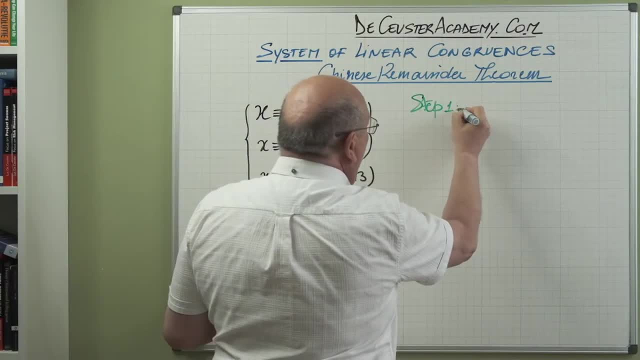 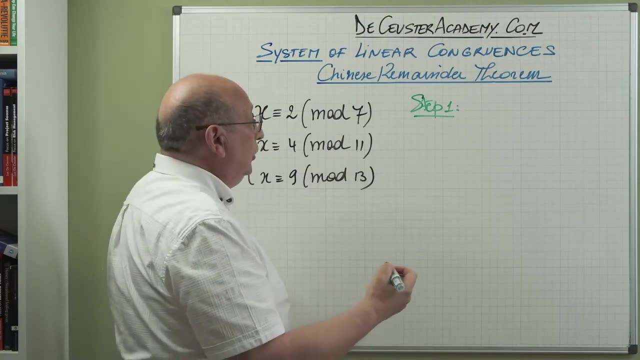 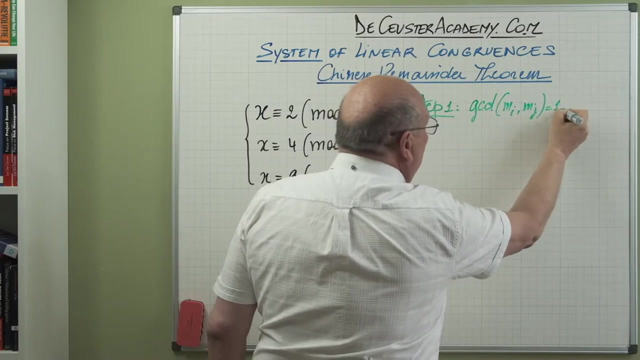 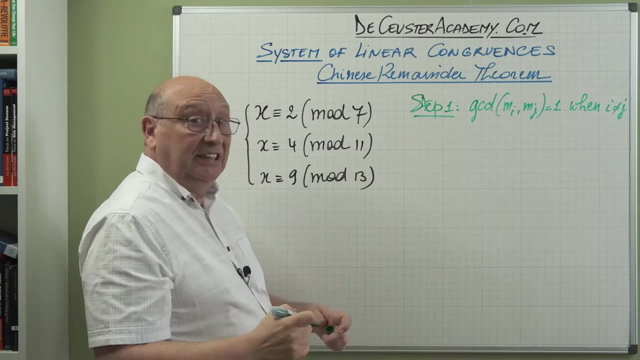 step 1, we have to verify if those moduli are relatively prime. So it means that we have to verify the GCD of M, i, M. j is equal to 1 when i is not equal to j. Now, in this case it's very easy, because the numbers 7,, 11 and 13 are special numbers. 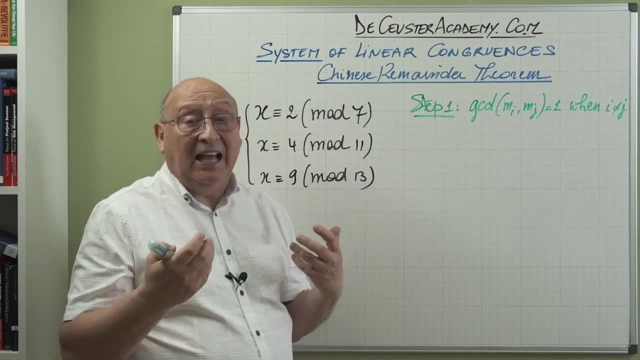 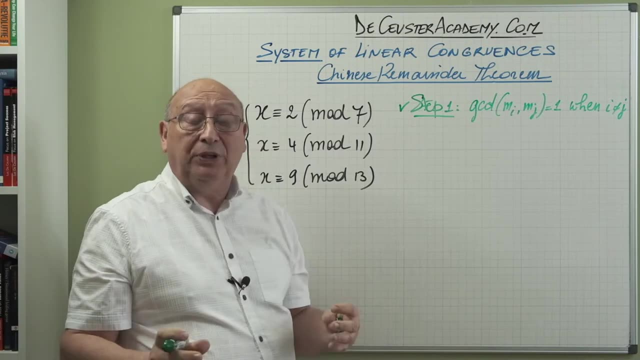 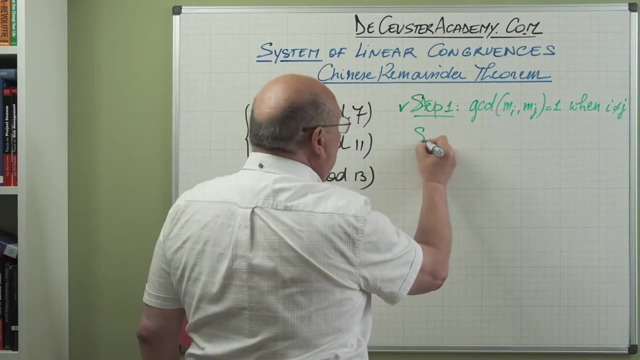 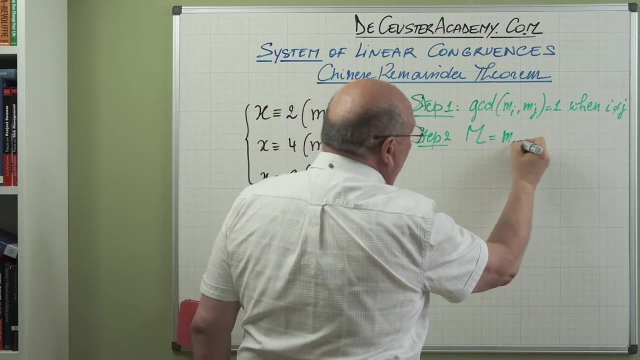 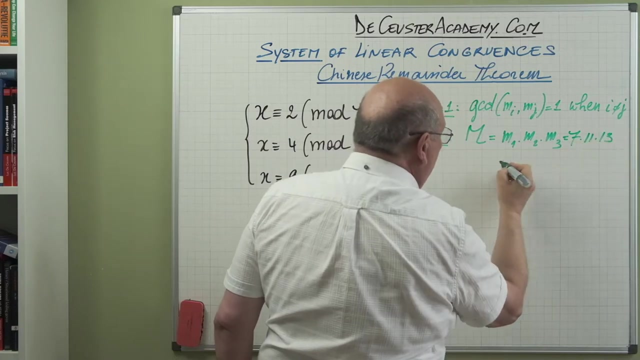 They're all prime numbers, so they always have a GCD which is equal to 1.. So this is confirmed, which means we have one unique solution for this problem. The second step, step 2, we have to find M, M, which is M1 times M2 times M3, which is in fact 7 times 11 times 13, and when you calculate this, 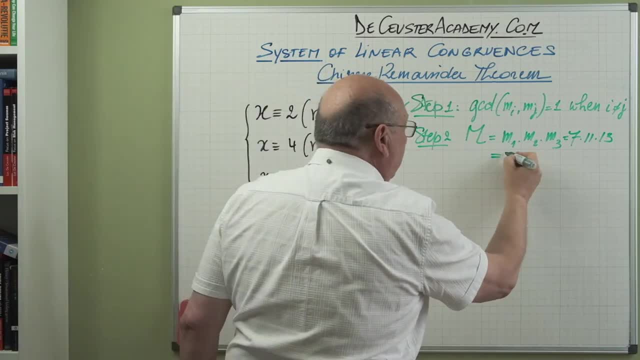 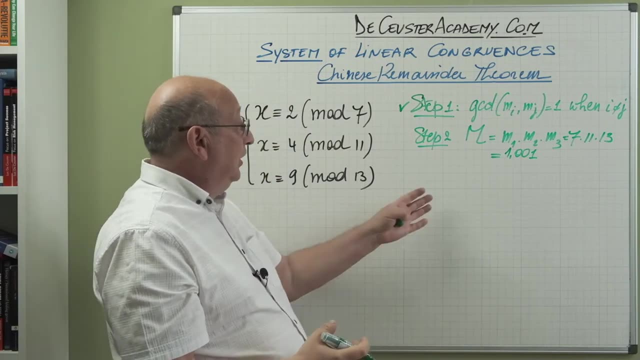 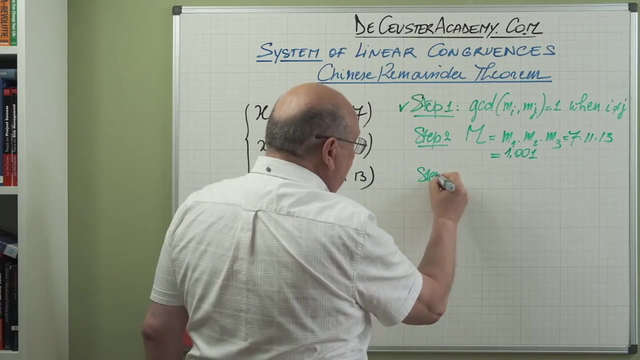 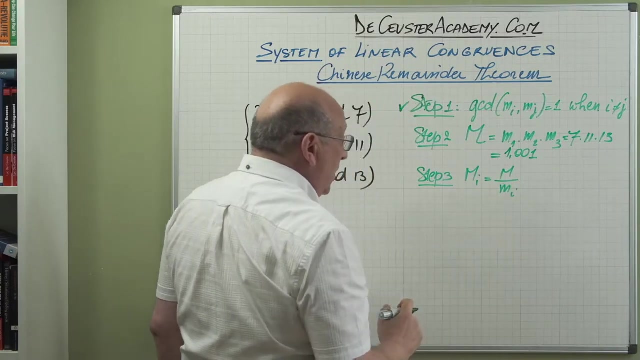 this will be equal to 1001.. So the solution we will find X will be equivalent modulus 1001.. So that's finished. The next step- step 3, is finding the big MI, which is M divided by MI. So we find big M1, which is equal to. 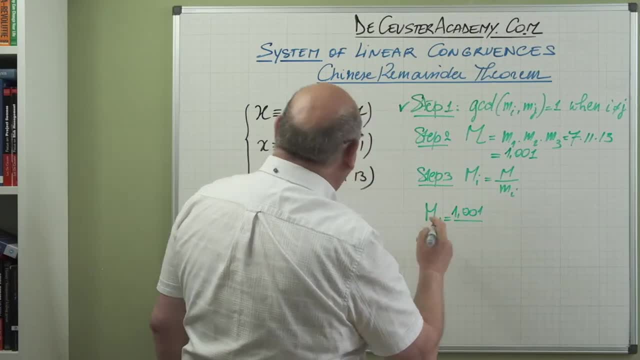 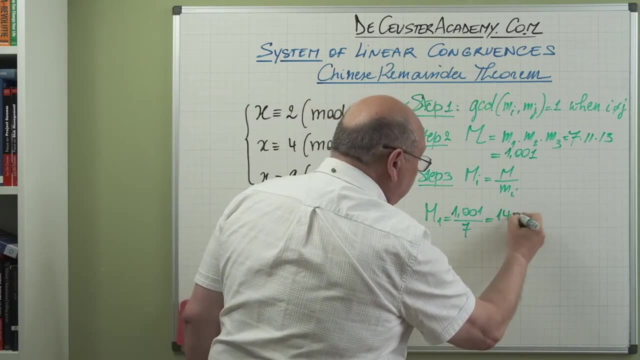 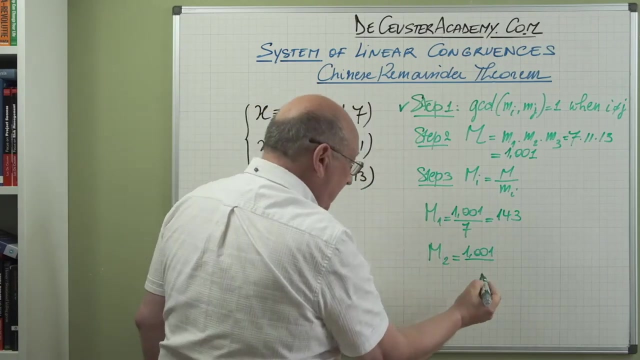 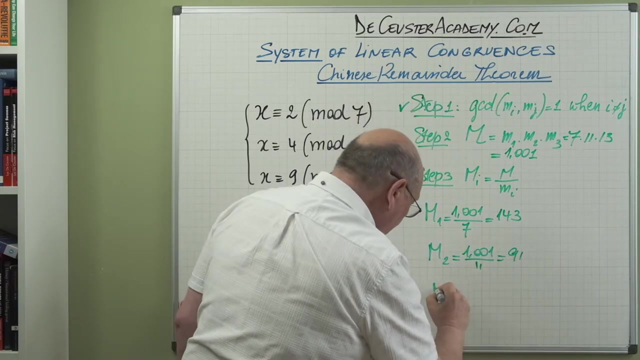 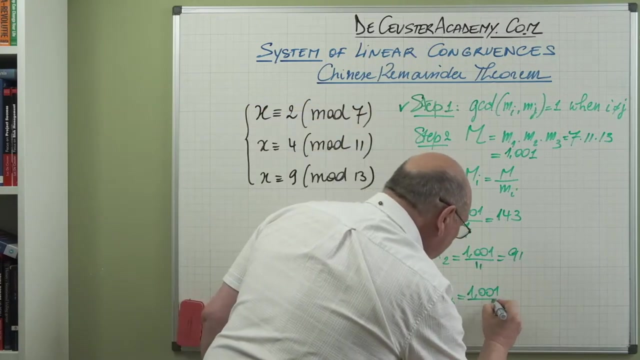 1001 divided by 7, which gives us the number 143.. Then we find M2, it's 1001 divided by 11, which is is equal to 91, and finally we have entry, which is equal to 1001 divided by 13. 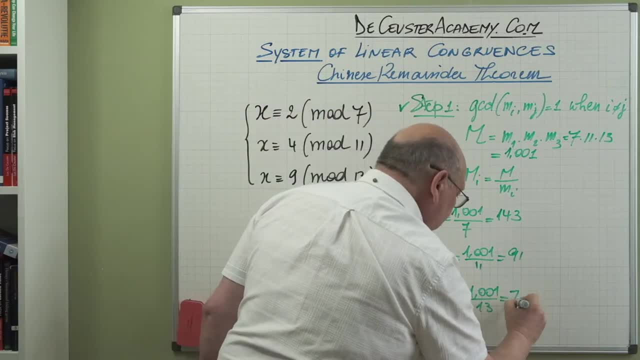 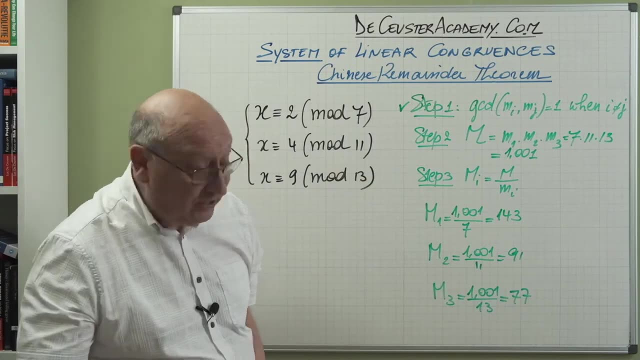 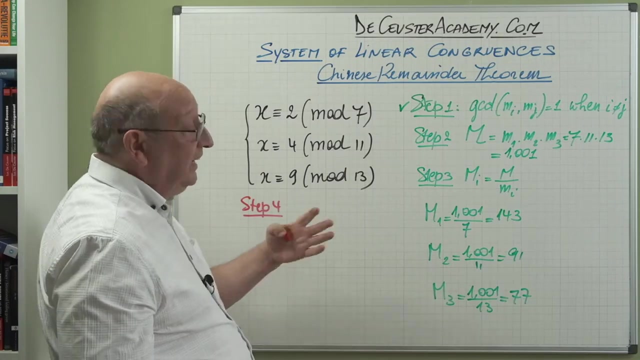 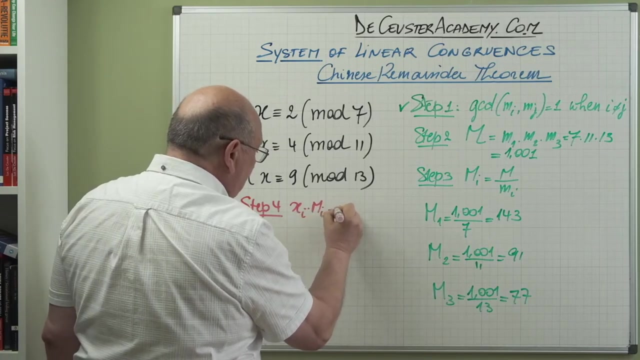 which is equal to 77 based on those equations. because based on the elements that we find here, we can write in step 4 the equations to find X 1, X 2 and X 3. so here we can write: X I times MI is congruent with 1 modulus MI. when we look 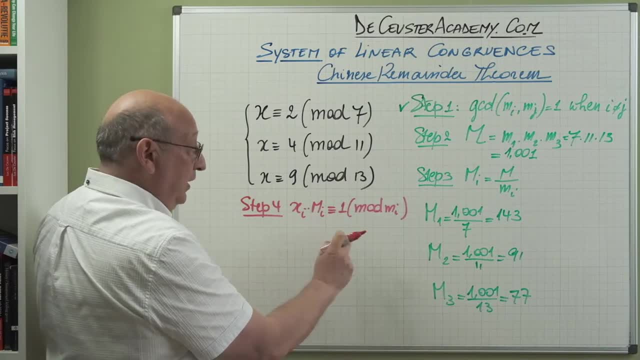 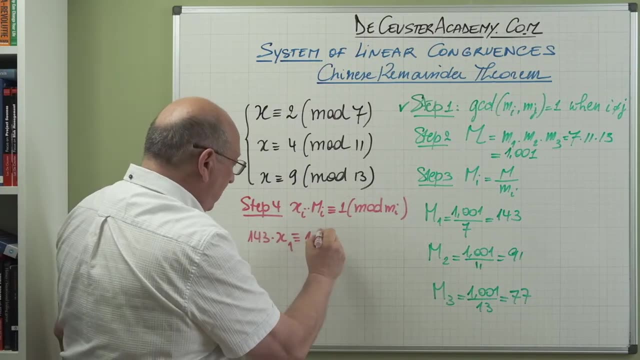 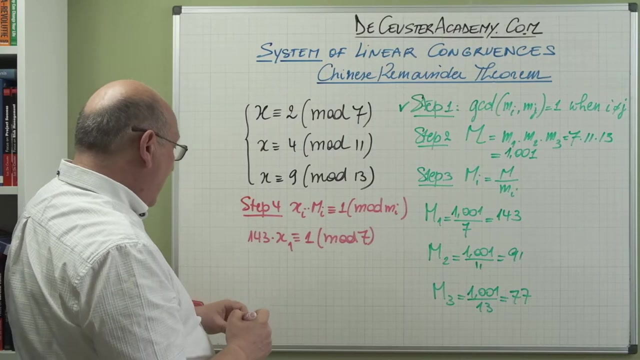 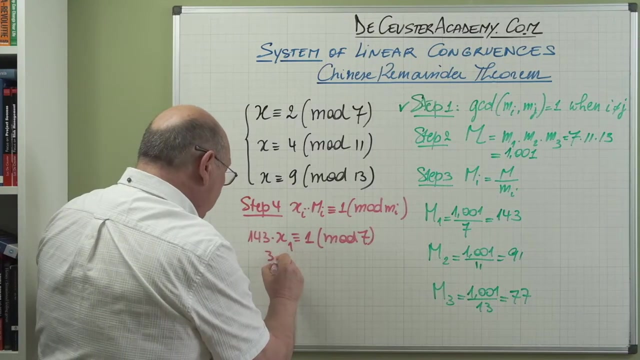 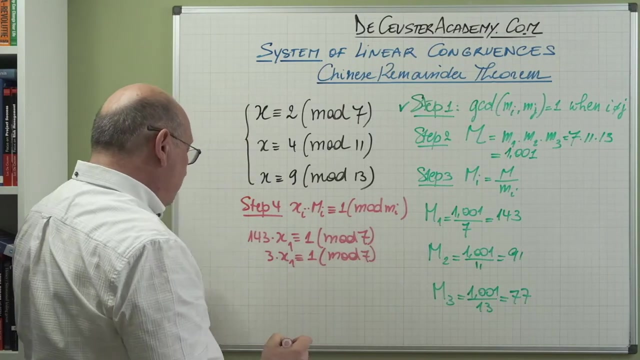 at the first equation we have X, 1 and 1, so we have 143 times X. 1 is congruent with 1 modulus 7. now we can rewrite this as 143 modulus 7 is the same as 3 times X. 1 is congruent with 1 modulus 7. now we have to find the modular inverse of 3. 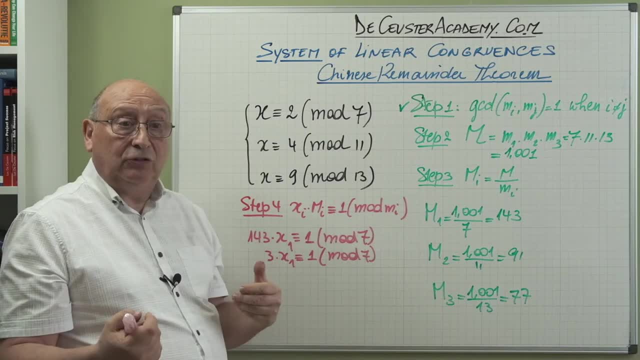 modulus 7. now, when we look at this, it's very easy to find the inverse of 3 modulus 7. now, when we look at this, it's very easy to to find the inverse of 3 modulus 7. now, when we look at this, it's very easy to find it because when we multiply both sides. 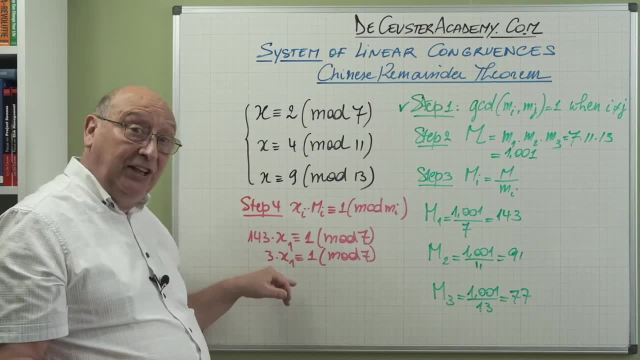 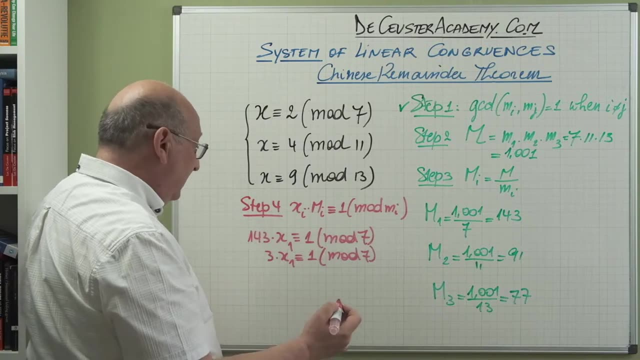 to find it. because when we multiply both sides to find it. because when we multiply both sides with 5, 5 times 3 is 15. 15 modulus 7 with 5, 5 times 3 is 15. 15 modulus 7 with 5, 5 times 3 is 15. 15 modulus 7 is in fact equal to 1. so we find here it's: 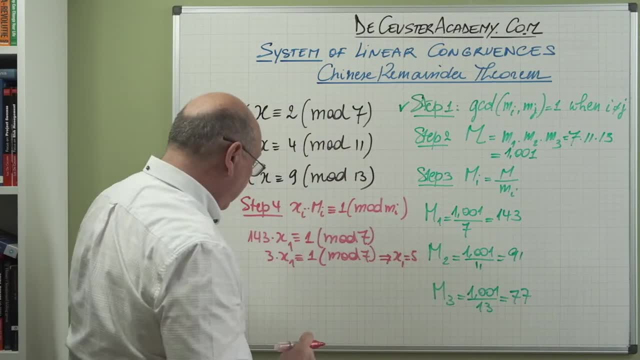 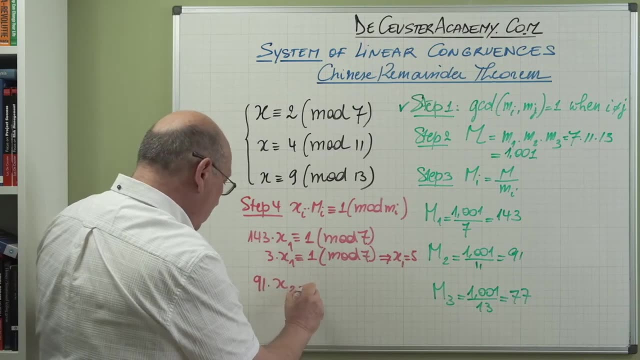 is in fact equal to 1. so we find here it's is in fact equal to 1. so we find here it's: 1 is 5. the second equation is 91: 1 is 5. the second equation is 91: 1 is 5. the second equation is 91 times X, 2 is congruent 1 modulus 11. we. 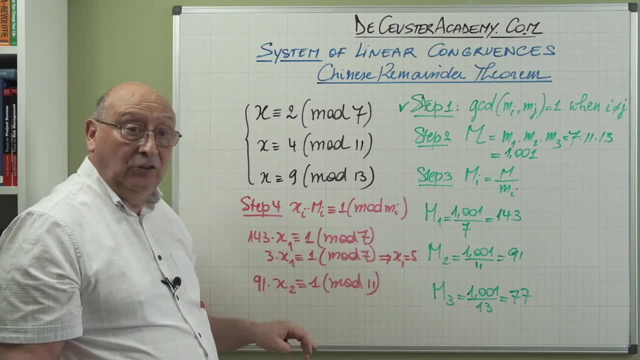 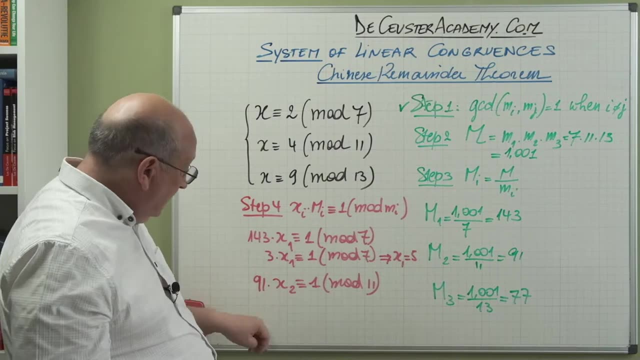 times X: 2 is congruent 1 modulus 11. we times X: 2 is congruent 1 modulus 11. we can rewrite this: 11 and 91. we can say: can rewrite this 11 and 91. we can say: can rewrite this 11 and 91. we can say that basically this becomes also 91- 11. 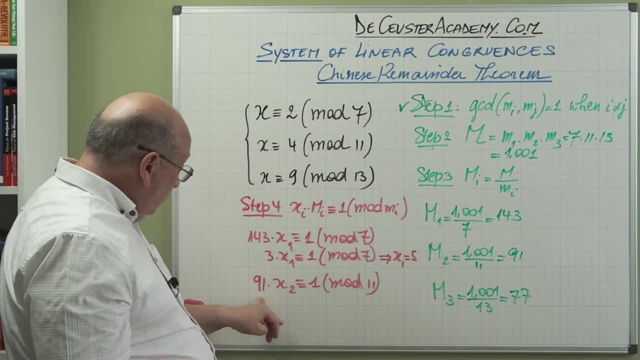 that basically this becomes also 91- 11, that basically this becomes also 91. 11 times 8 is 88, so we have 3. 91 is 3. 8 times 8 is 88, so we have 3: 91 is 3- 8. 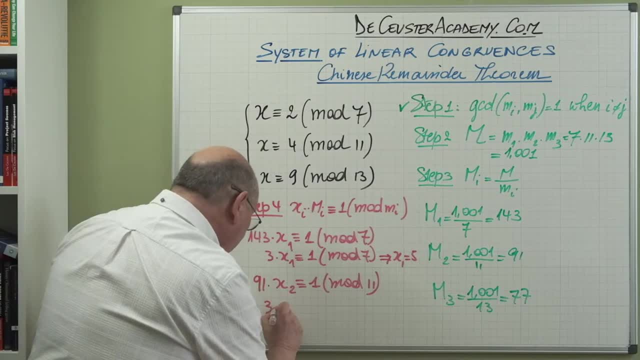 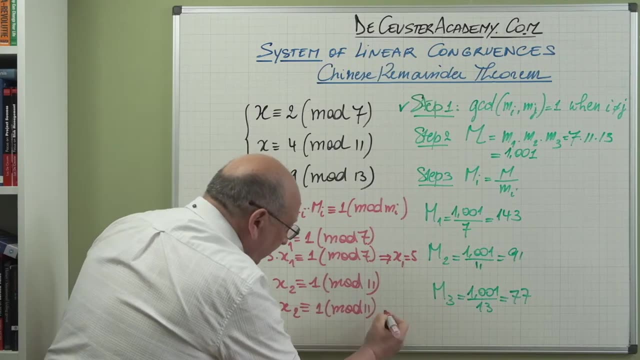 times 8 is 88, so we have 3, 91 is 3, 8 times 11 plus 3. so we find here 3 X 2 is times 11 plus 3, so we find here 3 X 2 is times 11 plus 3. so we find here 3 X 2 is congruent with 1 modulus 11, and we see: 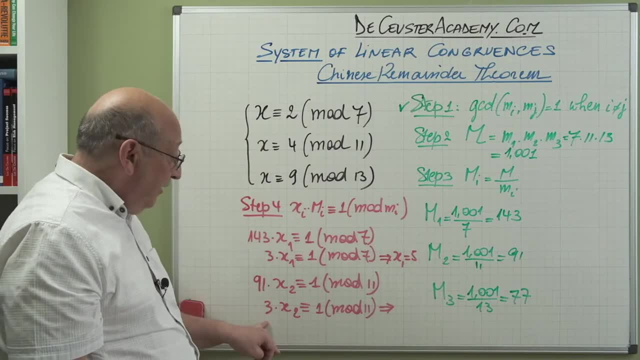 congruent with 1 modulus 11. and we see congruent with 1 modulus 11. and we see: when we multiply both sides with 4, we, when we multiply both sides with 4, we, when we multiply both sides with 4, we have 12, and 12 is equal to 11 plus 1. so 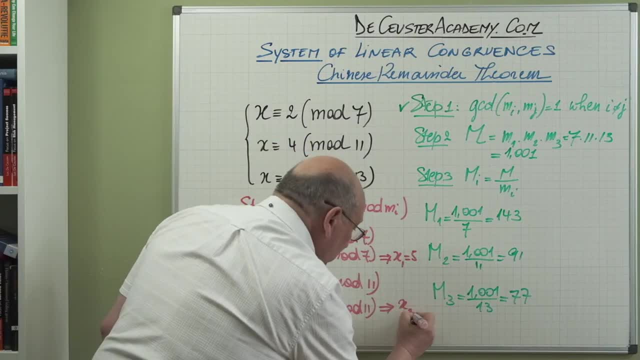 have 12 and 12 is equal to 11 plus 1. so have 12 and 12 is equal to 11 plus 1. so the modulus is 1 and we can say that X. the modulus is 1 and we can say that X. 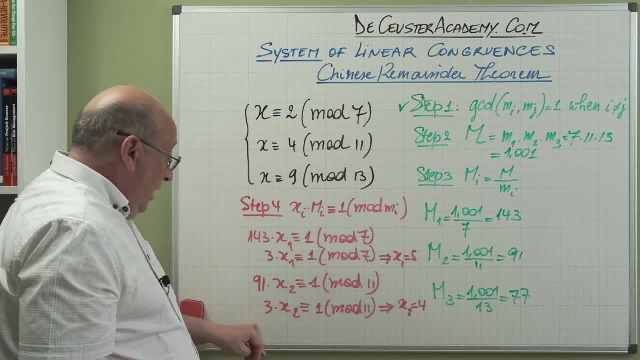 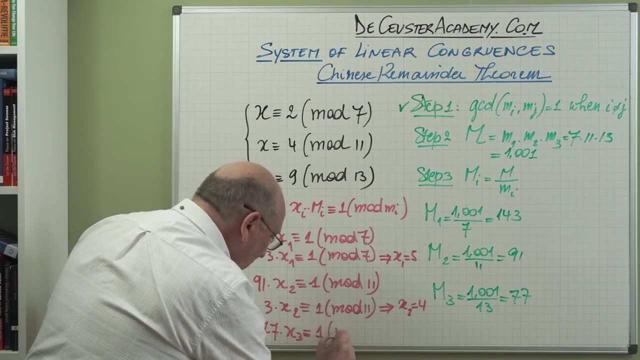 the modulus is 1 and we can say that X, 2 is equal to 4. the last one we have, 7, 2 is equal to 4. the last one we have, 7, 2 is equal to 4. the last one we have, 7, 7, X, 3 is congruent with 1, modulus 13 now. 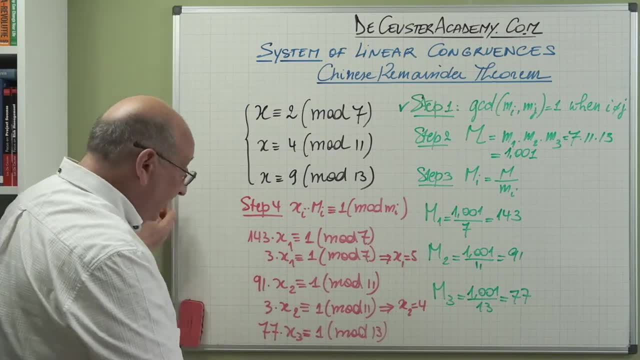 7, 7 X 3 is congruent with 1 modulus 13. now, 7, 7 X 3 is congruent with 1 modulus 13. now, what we can do here 77, 77, 77 is what we can do here, 77, 77, 77 is. 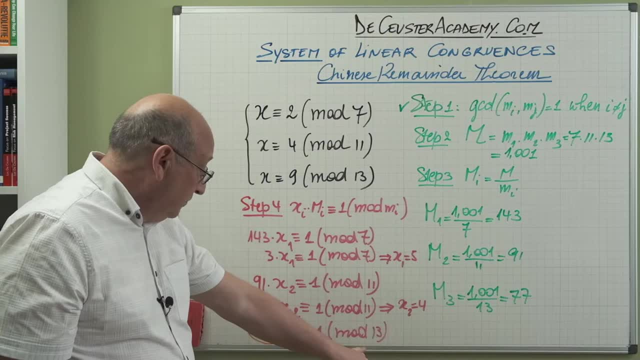 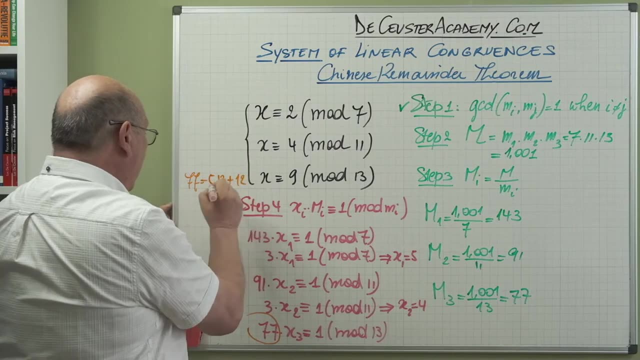 what we can do here. 77, 77, 77 is equal to when we look at it 5 times 13 plus 12, equal to when we look at it 5 times 13 plus 12, equal to when we look at it 5 times 13 plus 12, and with: 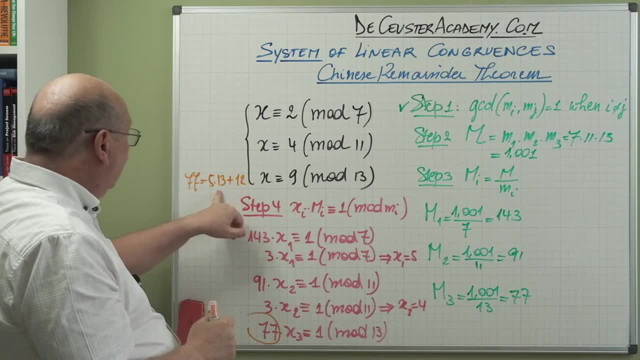 and with and with. find here: this is 50. this is 65 plus 12. find here: this is 50. this is 65 plus 12. find here: this is 50. this is 65 plus 12 is 77. so we find here 12 X 3 is. 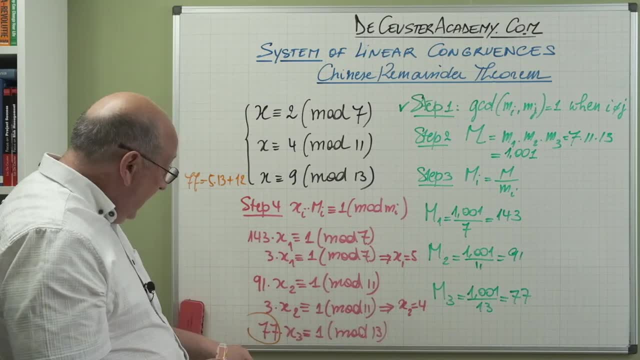 is 77, so we find here: 12 X 3 is is 77, so we find here: 12 X 3 is equivalent with 1 modulus 13 and we can equivalent with 1 modulus 13 and we can equivalent with 1 modulus 13 and we can find that the modular inverse in that 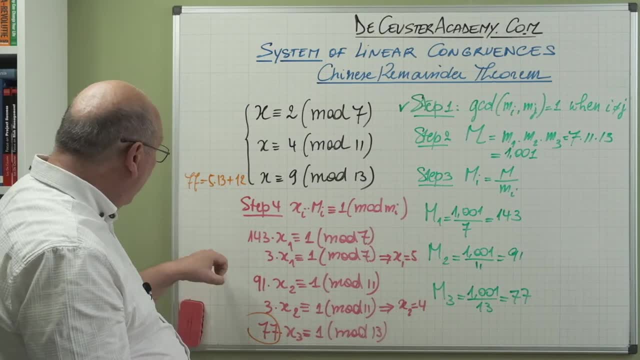 find that the modular inverse in that find that the modular inverse in that case is 12. so we multiply both sides, case is 12. so we multiply both sides, case is 12. so we multiply both sides with 12. 12 times 12 is 144, which is. 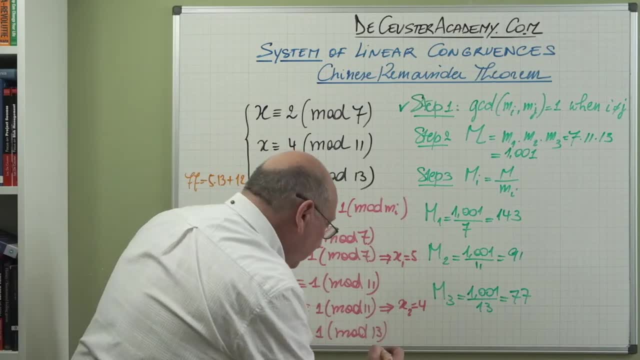 with 12. 12 times 12 is 144, which is with 12. 12 times 12 is 144, which is: modulus 13 equal to 1. modulus 13 equal to 1. modulus 13 equal to 1. so we can say that X 3 is equal to 12. so 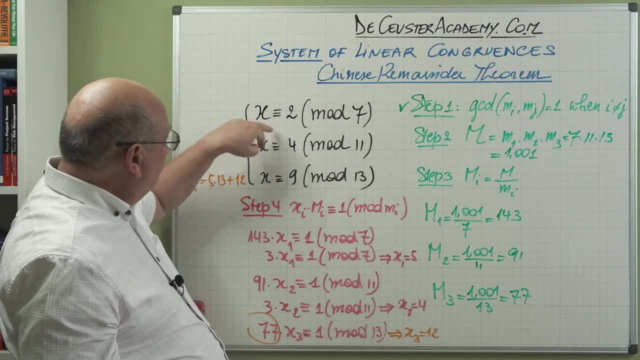 so we can say that X 3 is equal to 12. so so we can say that X 3 is equal to 12. so, basically, what we found here, we found, basically what we found here. we found basically what we found here we found we have the terms b1, b2, b3, we have m1, m2. 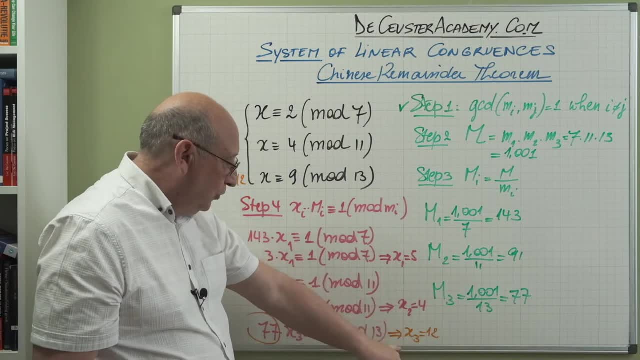 we have the terms b1, b2, b3. we have m1, m2. we have the terms b1, b2, b3, we have m1, m2 and 3 and we have each one x2 and x3 and 3 and we have each one x2 and x3. 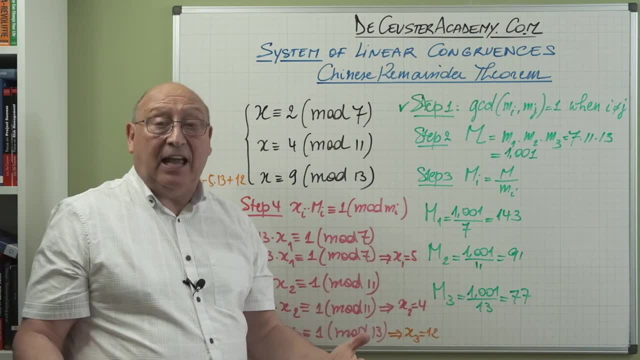 and 3, and we have each one x2 and x3. now we can put all the information in a. now we can put all the information in a. now we can put all the information in a table and calculate the value of X table and calculate the value of X. 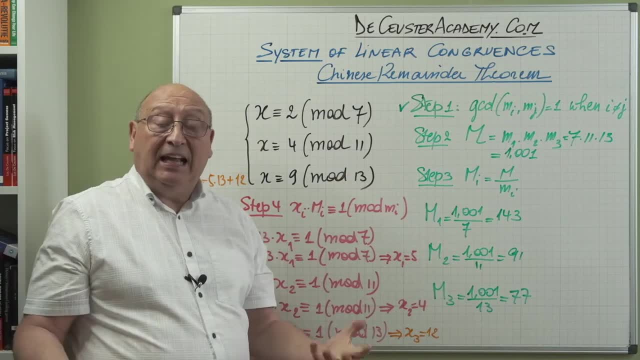 table and calculate the value of X modulus 1001 and see what the final modulus 1001 and see what the final modulus 1001 and see what the final result is. what is the X value? that result is: what is the X value? that result is: what is the X value that complies with these three linear 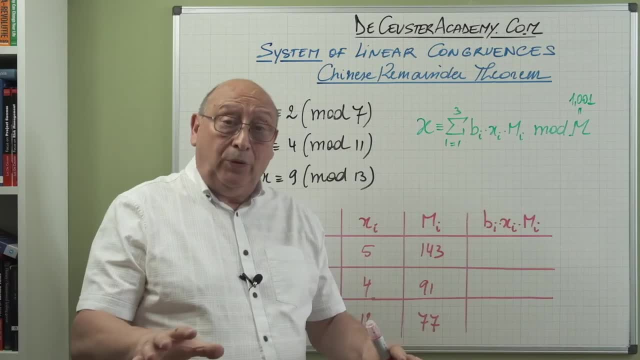 complies with these three linear complies with these three linear concurrences simultaneously. now we can concurrences simultaneously. now we can concurrences simultaneously. now we can put everything in a table. so we have the put everything in a table. so we have the put everything in a table. so we have the coefficients bi, 2, 4 & 9, we have the. 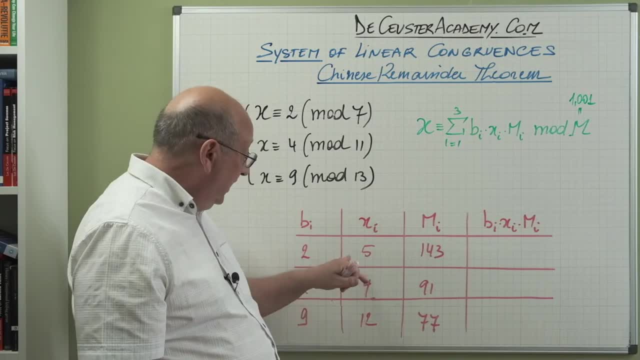 coefficients bi 2, 4 & 9. we have the coefficients bi 2, 4 & 9. we have the coefficients X I we found in the previous coefficients X I we found in the previous coefficients X I we found in the previous calculation being 5, 4 & 12 and the mi. 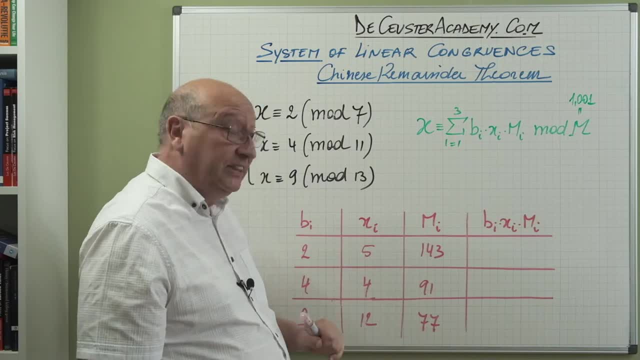 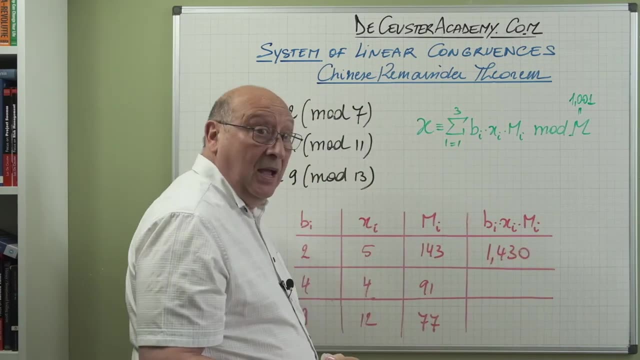 calculation being 5, 4 & 12 and the mi calculation being 5, 4 & 12 and the mi big mi 143, 91 and 77. so when we big mi 143, 91 and 77, so when we big mi 143, 91 and 77, so when we multiply those, we win. we find 1430. the 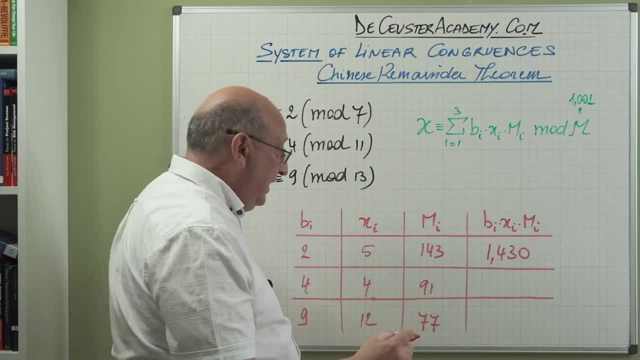 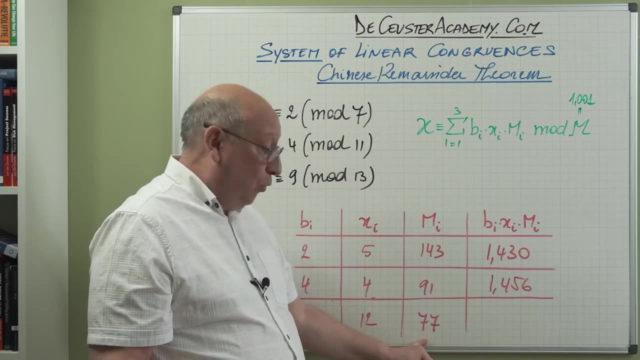 multiply those we win: we find 1430. the multiply those we win: we find 1430. the second one 4 times 4 times 91 is 1456. second one 4 times 4 times 91 is 1456. second one 4 times 4 times 91 is 1456. and the last one, 9 times 12 times 77. 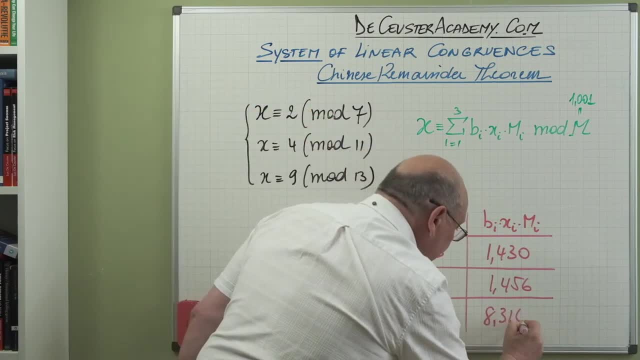 and the last one 9 times 12 times 77 and the last one, 9 times 12 times 77 is in fact 8316. when we put all of them is in fact 8316 when we put all of them is in fact 8316 when we put all of them together. 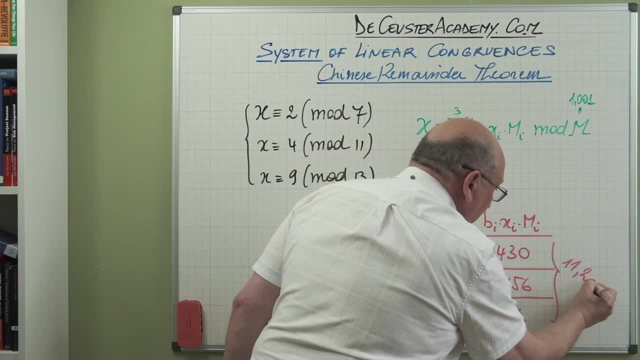 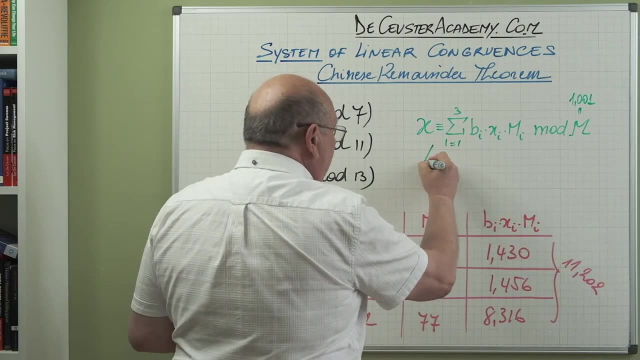 together. together, we find 11,000 202, we find 11,000 202, we find 11,000 202. modulus 1001, so we can complete this. now we modulus 1001, so we can complete this. now we modulus 1001, so we can complete this. now we can say that X is equal to 11,000 202.